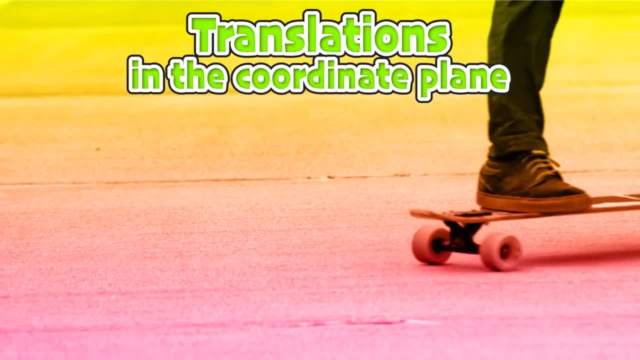 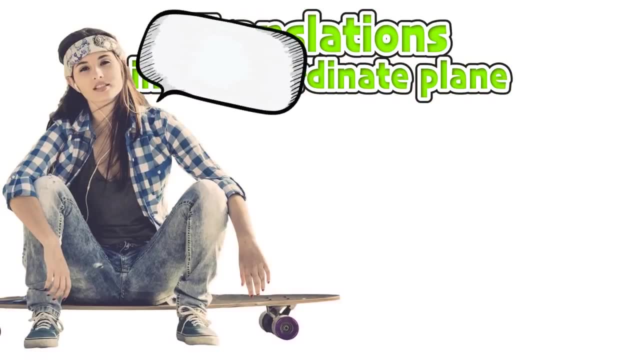 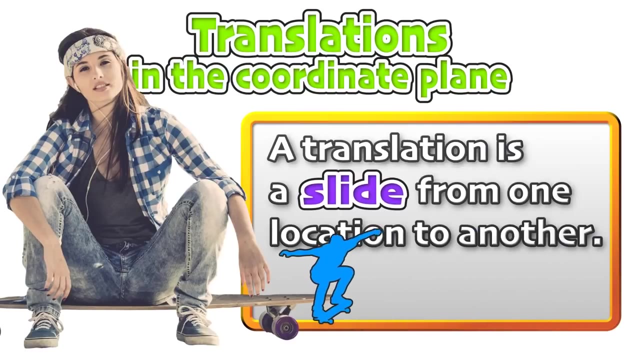 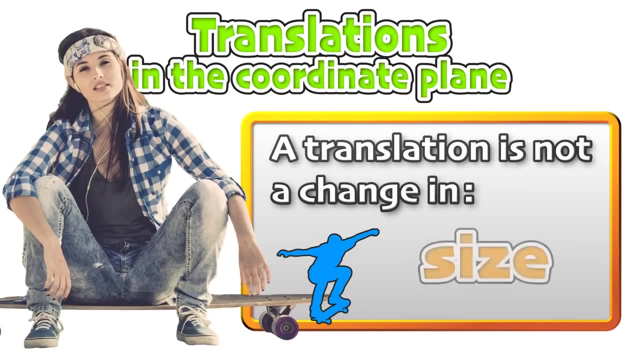 We'll start this lesson off by watching a skateboard sliding along the pavement, Much like Jennifer on her skateboard. a translation is a slide from one location to another. A translation is not a change in size and a translation is not a change in orientation. 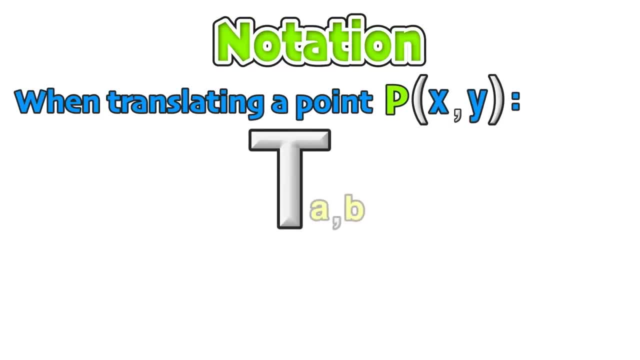 When translating a point P with coordinates, we can use the capital T notation. Our point P with coordinates is translated to the new point P' Notice that the A and B values correspond with the X and Y coordinates of the point P as it's translated to P'. 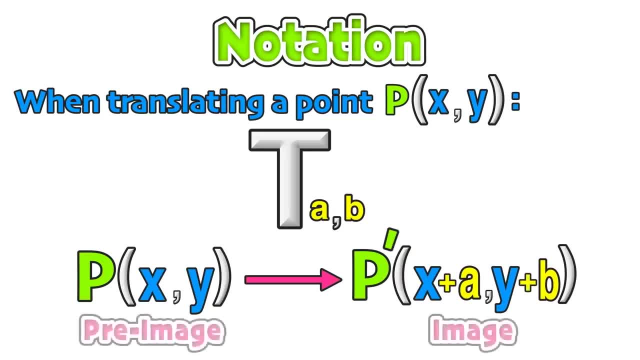 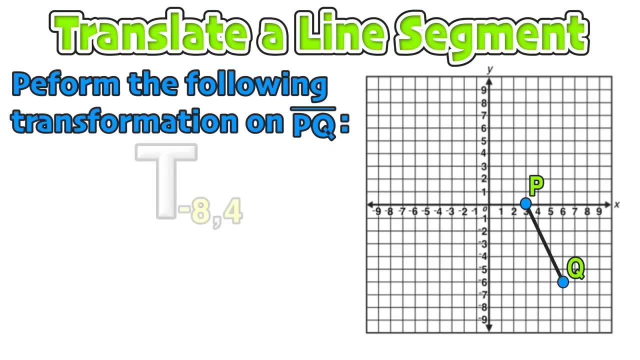 By applying these values we can find the coordinates of the image P'. Let's start our first example by performing the following transformation on line segment PQ. We can start by writing down the coordinates of the endpoints of PQ with P at and Q at. 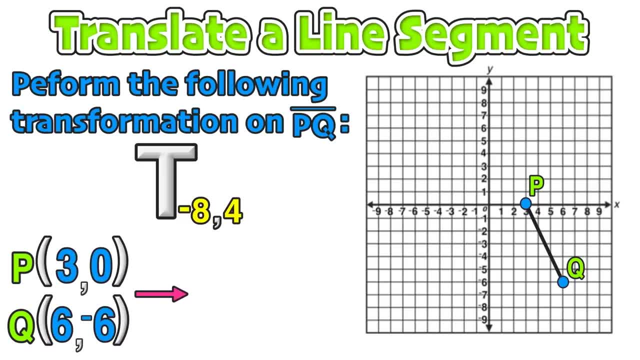 Now, since this line segment is being translated, we know that P' and Q' will have different coordinates than P and Q. Since our first value is a negative 8,. we'll subtract 8 from both X values and remember that the X axis is horizontal, so a negative 8 for X means 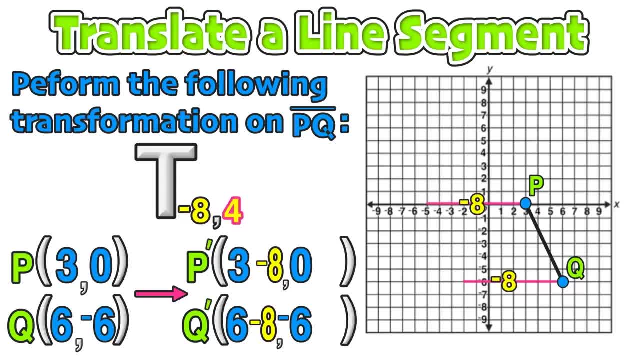 moving to the left, 8 spaces. Our second value, positive, 4, corresponds with the Y values. so we will add 4 to each Y value And that is the same thing as going up 4 units. And now that we have our path laid down, we can look at the graph and visualize that line. 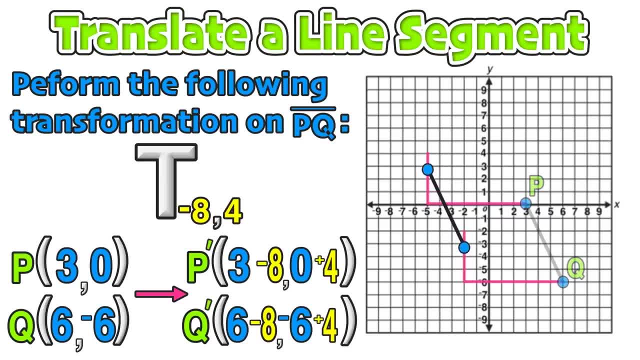 segment PQ being translated to its new location at P' Q' Finally, we can verify our final coordinates by finding the first X value: 3 minus 8, is negative, 5,, 0 plus 4 is just positive 4, and now for Q', 6 minus 8 is equal to 4.. 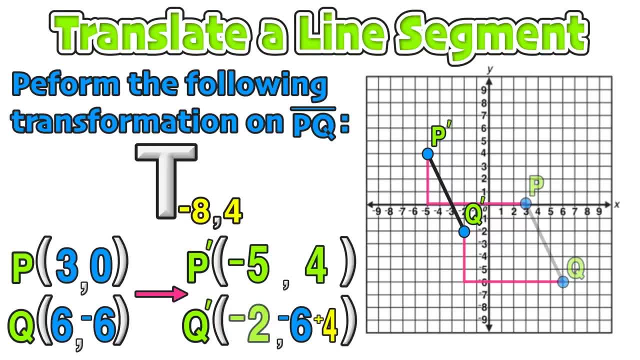 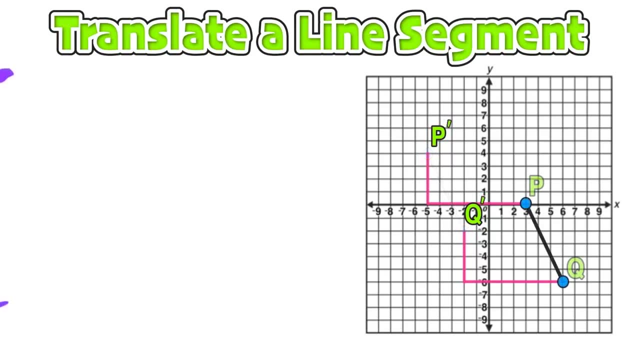 Q' 6 minus 8 is equal to negative 2, and the final coordinate, negative 6 plus 4 is equal to negative 2.. Notice that these points correspond with our graph for the image of line segment P' Q' Now we can visualize and conceptualize just what it means for a line segment to be translated. 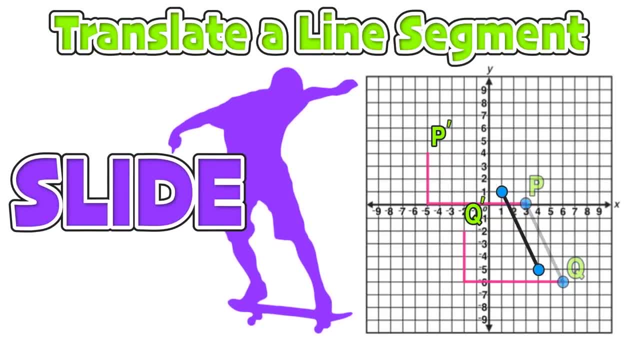 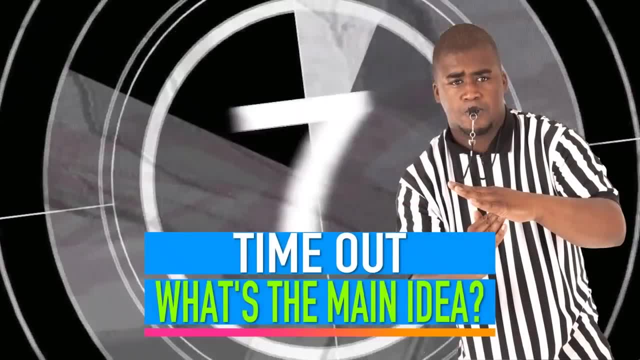 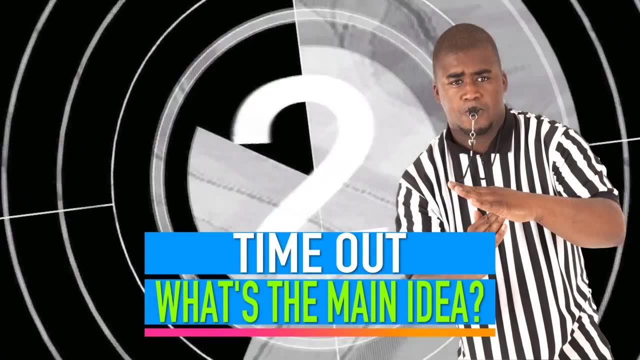 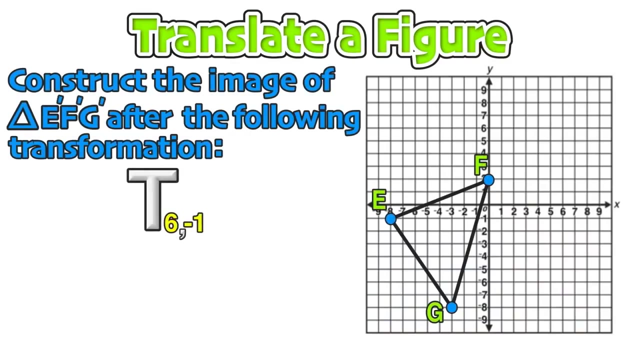 by sliding it from one location on the coordinate plane to another. For our last example, we are going to construct the image of triangle E', F' G' after the following transformation. We'll start off by writing down the coordinates of the vertices of triangle E, F, G To find: 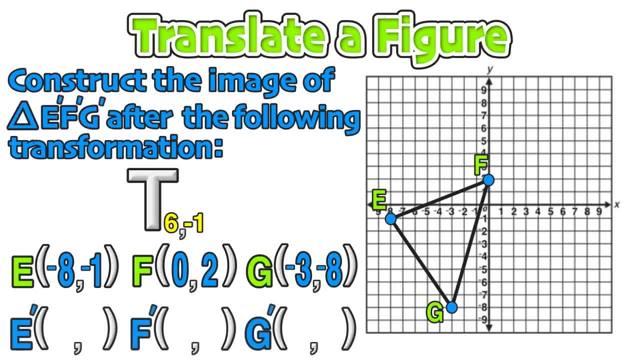 the coordinates of E' F' and G' we'll start by applying the values of the translation. The X value is 6, so we're going to add 6 to all of the X values in each coordinate. Positive 6 calls for us to slide 6 units to the right horizontally along the X axis. 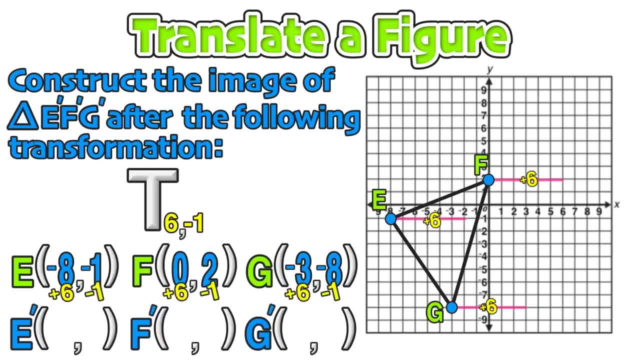 Next is the Y value of negative 1.. We are going to subtract 1 from all of the Y coordinates On the graph. negative 1 means to move down vertically 1,, 2,, 3,, 4,, 4,, 5,, 6,, 6,, 7,, 8,, 9,, 10,. 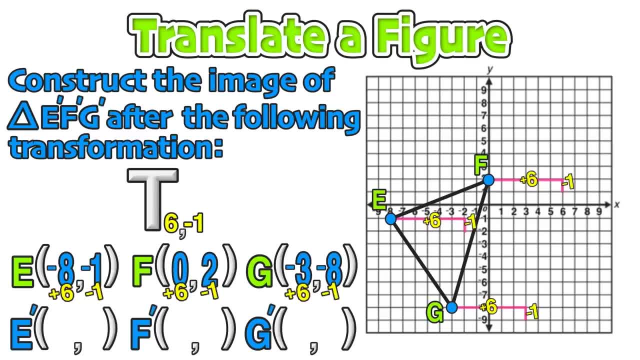 and 10 units along the Y axis. Now to verify the coordinates of E', F' and G' We start by adding 6 to each X Coordinate and that will give us the new X coordinate of E' F' and G' We'll do the same thing with the Y coordinates, by subtracting 1 from each to get those new. 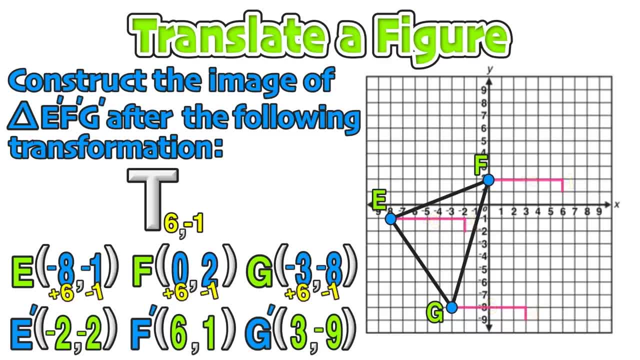 Y coordinates. Now we can look at the graph and visualize the original image being translated to the right, 6 units and down: 1. To its new location at E', F', G' You now know your protocol And we can see that our points E' at, F' at and G' at all correspond.